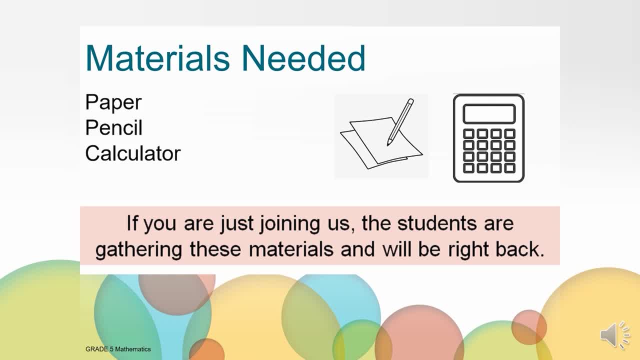 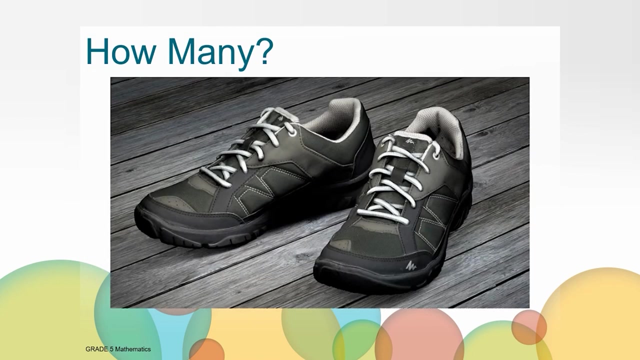 in previous lessons. you'll need some paper, something to write with and a calculator. Go ahead and gather your materials and come right back. Take a look at this picture. How many, How many? what you might be asking? Well, that's part of this routine. You can choose anything in this picture and tell. 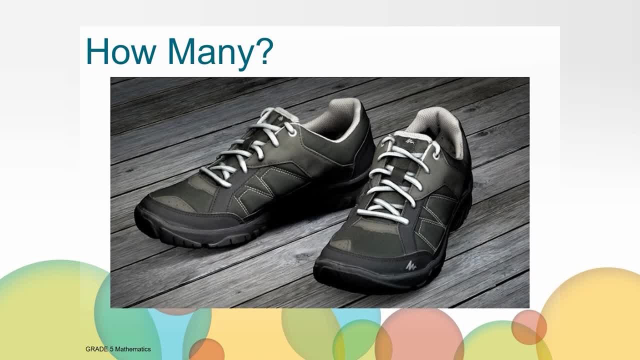 us how many, as long as you can prove it, Turn and tell someone near you, or write down your thoughts, the number of logos on the shoes, or maybe two, as in two shoelaces? did you say three, as in the number of logos on the shoes? 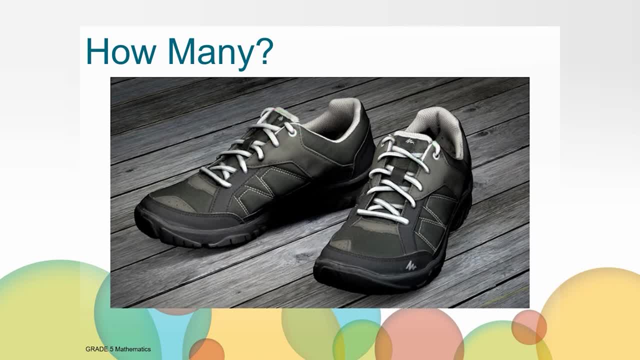 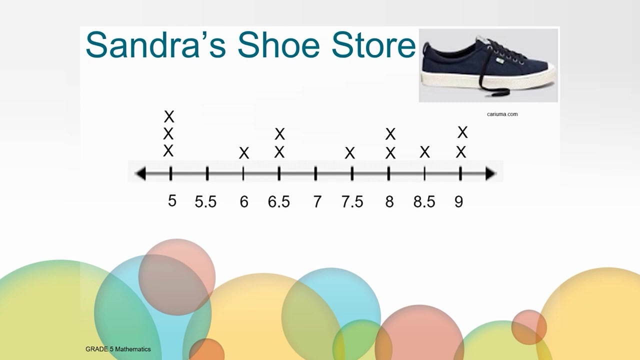 or maybe you counted 12, as in the number of planks of wood on the floor, you may have counted other things as well. Let's look at this data from Sandra's shoe store. These are the sizes of the last 12 pairs of these black. 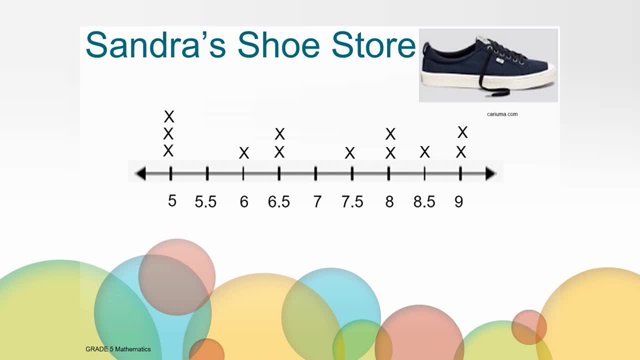 shoes sold at Sandra's. The owner, Sandra, wants to order more of these popular shoes. She's not sure whether to use the mean, median or mode to find out what the most popular size is. Help her out by taking about two minutes to find the. 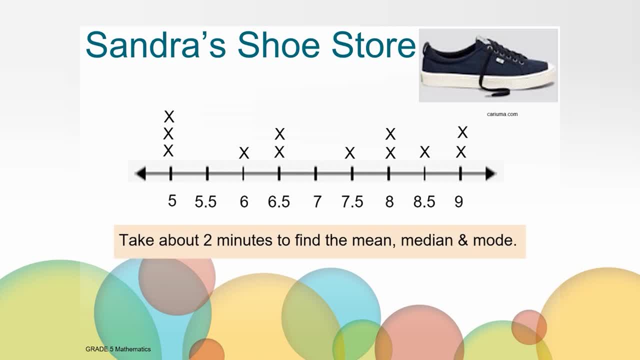 mean median and mode of this data and then select which is the best representation of what she should order and then select which is the best representation of what she should order. and then select which is the best representation of what she should order. 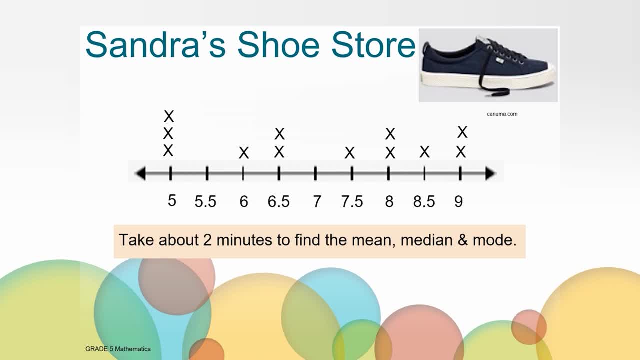 If you remember, it will take you about 40 seconds to find each pair of your favorite shoes. That's right. 3defined 10 können tidak: 31, 31, 33, 34, 35, 36, 37, 38, 39, 40. 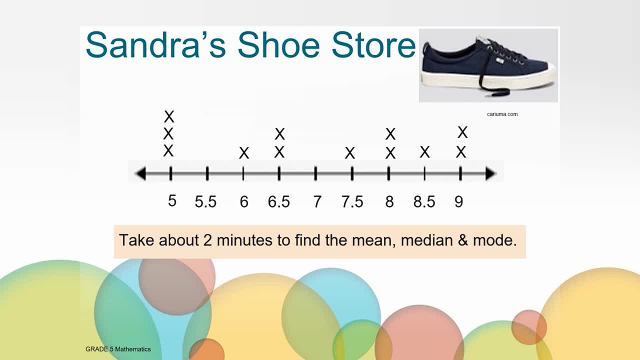 41, 42, 42, 53, 43, 43. Thank you. Okay, did you get seven for the mean and for the median and then five for the mode. So which size is the best representation of what Sandra should order? Well, this is tough because two of the measures of center we calculated- the mean and the median- both show that seven is the middle value or the average. 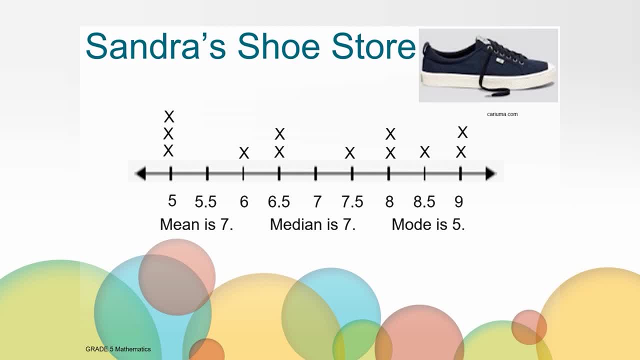 But for ordering shoes is the average the best measure of center. We should probably look at what the median is. We should probably look at what the most popular shoe size is so that we can reorder that size. The measure of center that represents the most popular piece of data is the mode. 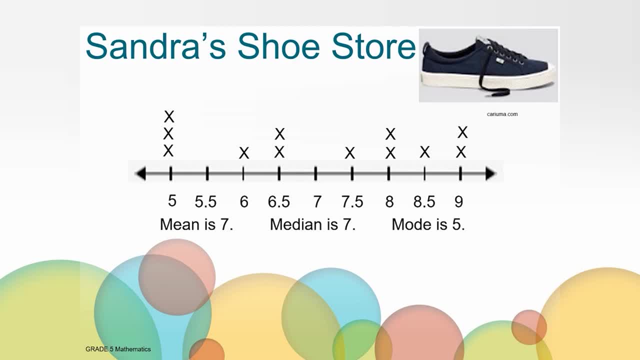 So in this case the mode is probably the best indicator of what Sandra should reorder. After size five, there are three other shoe sizes that are equally popular: Six and a half, eight and nine. Does this mean that Sandra will sell these sizes? 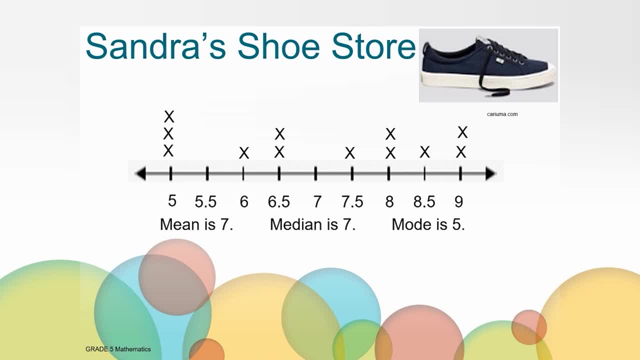 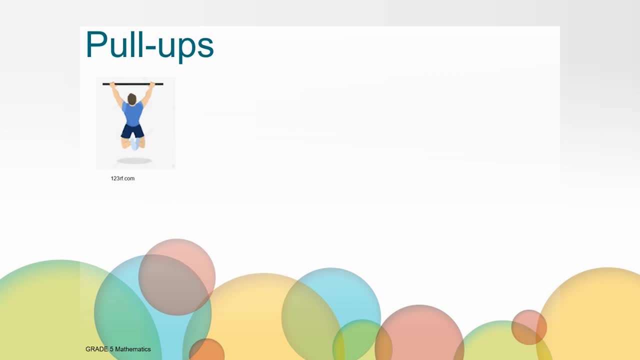 Not necessarily, but mode seems to be a better measure of center for this context. Now let's consider another context. Luis does some pull-ups every day, each week. Here is the data of how many pull-ups he did in the first week: The mean, median and average. 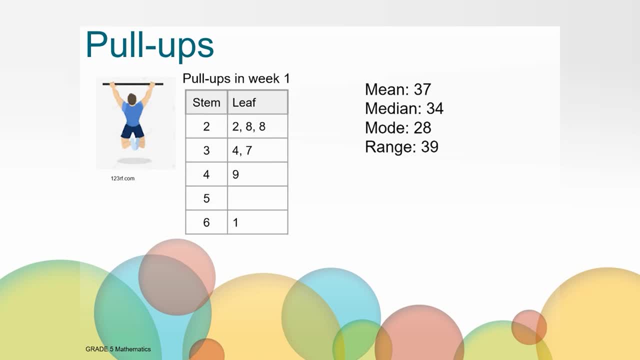 The median mode and range for the data set are also listed here. What do you notice and what conclusions can you make? Well, we can state some facts about the data. Like Luis did 28 pull-ups twice in the week. 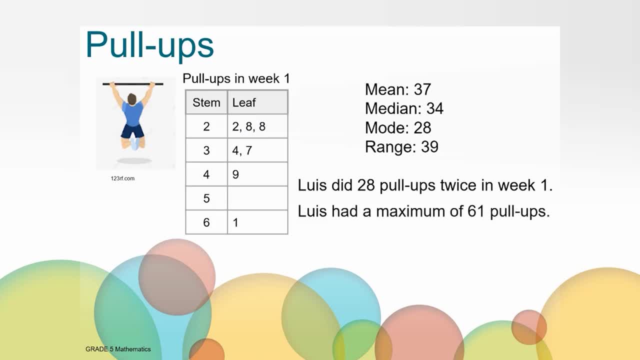 Or on one day Luis did 61 pull-ups, which was the most he did the whole week. Can we say that Luis improved in the number of pull-ups he did over the week? Well, since we don't know which number of pull-ups Luis did at the beginning of the week versus the end of the week, 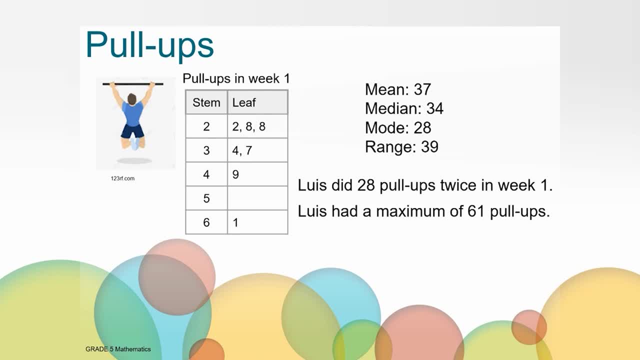 we can't really say that Luis did the most pull-ups he did over the week. We can't really answer that question. Data usually doesn't mean much on its own, but rather it takes on more meaning when you compare it to other data. 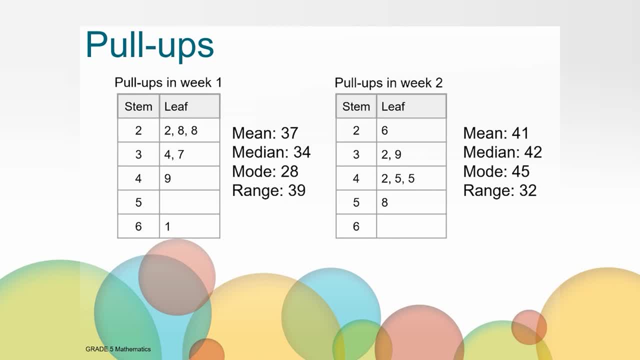 So let's look at some more data. Here's the data for the number of pull-ups Luis did in his second week. Think about what you notice. Take a minute to practice being a communicator by telling someone your thoughts or writing down some conclusions. 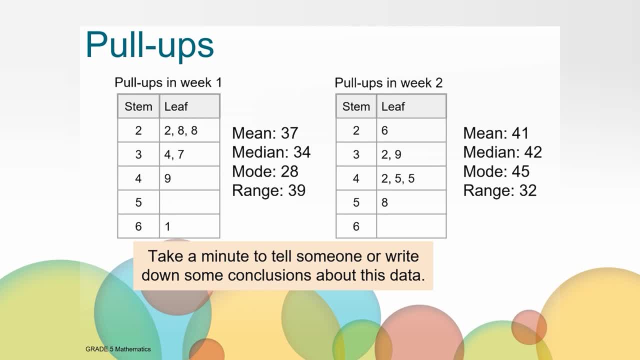 Here are some of the conclusions that you can make. You can get a little bit more information about what your thoughts are. with a search engine like me, It's important that you know how to process what you're saying, But most people don't have the ability to do so. 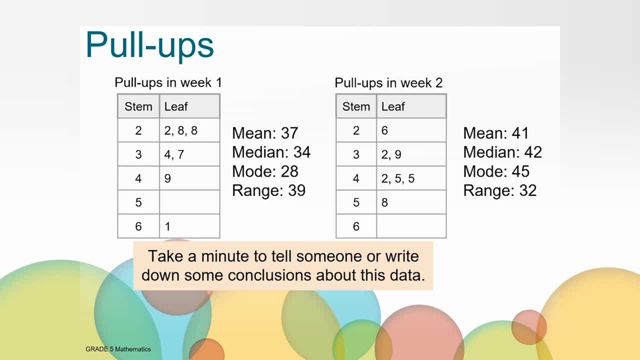 It's important to have a goal in mind too. Those goals will soon become a reality for everyone and everyone. Thank you. What did you make? by looking at this data, I noticed a few things. The range is less in week two than in week one. 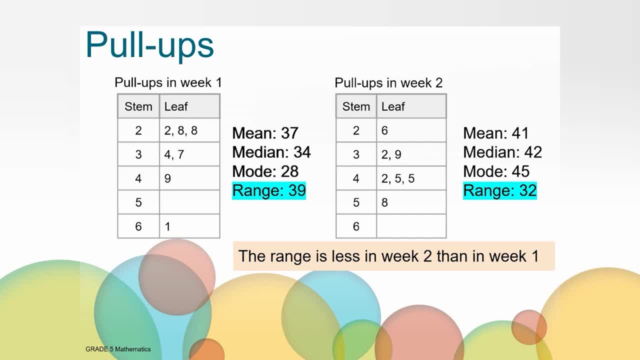 This means that the data values are actually closer to each other in week two and more spread out in week one. I also noticed the maximum number of pull-ups that Luis did in week one was higher than the maximum he did in week two. However, the minimum number of pull-ups that he did in week one. 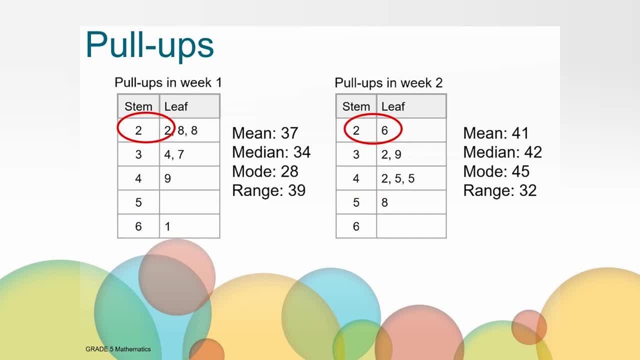 was lower than the minimum in week two. I also noticed that the mean median and mode were all higher in week two than in week one. So it seems that Luis is getting stronger and able to do more pull-ups each day. If Luis continues to work out in a week, 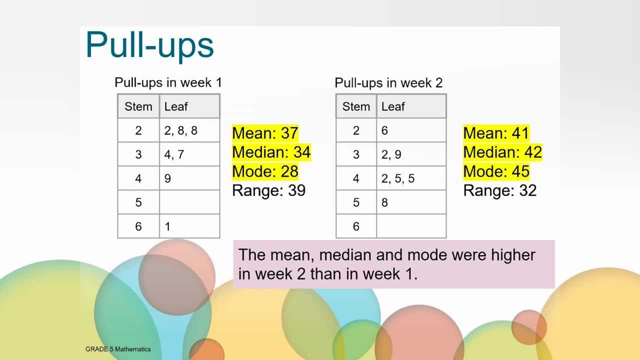 in a similar way every day. what might you expect the data for week three to look like? Maybe slightly higher data than week two? Well, we do know that oftentimes, when people exercise or practice consistently, they improve, whether that's in exercise or music or academics. 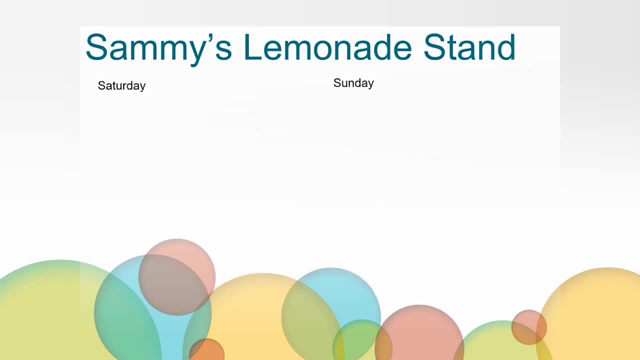 Make sure to work out theパンプ dealership. Kyle might even be one of some of these, and if you have a strong guessed question that they think, have them off, just like you tell me in the comments below. The portals for raussel and shovel are: 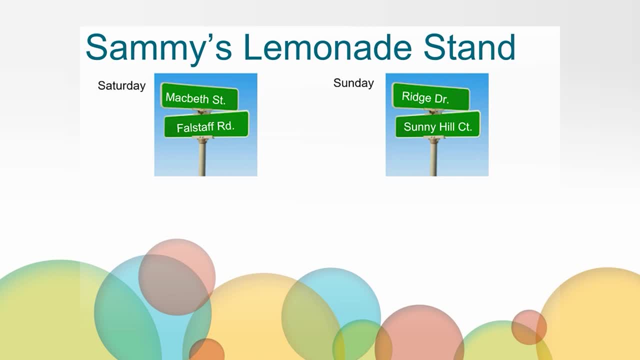 These are for customers- students- to have at home. These are for families to do their work. Keep in date as well afternoon to see which corner had better business. Well, he actually made the same amount of money on both days. He did take data of how many customers visited his 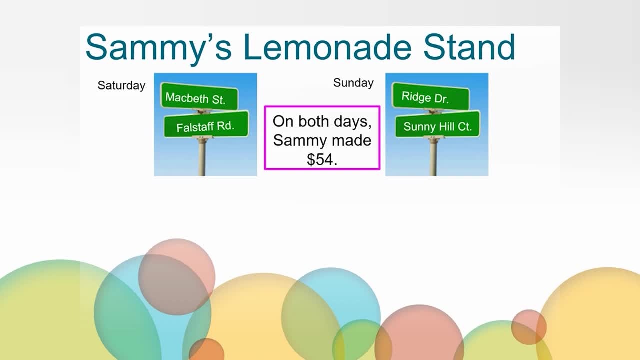 stand and how many cups of lemonade each customer bought. Then he figured out the mean median and mode for each day's sales. Although he ended up making the same amount of money, he wants your help to figure out at which corner he should. 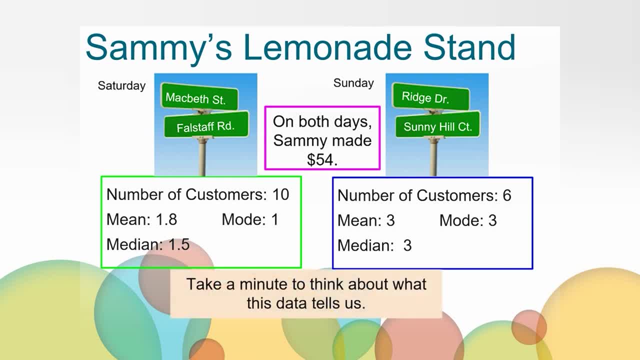 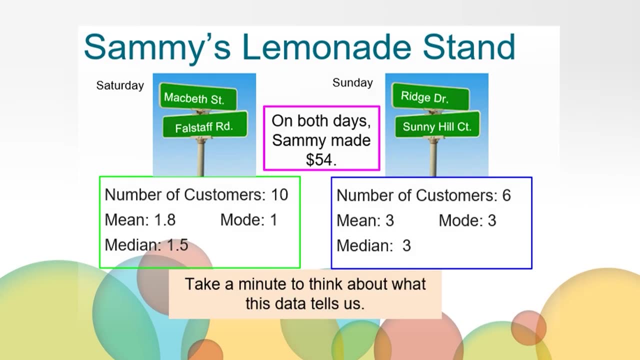 set up his stand in the future. Take a minute or so to think about what each of these measures of center, the mean, median and mode might tell us about Sammy and his customers. It's not going to be easy for the next 20,, 30,, 40,, 50, or 60 customers to get. 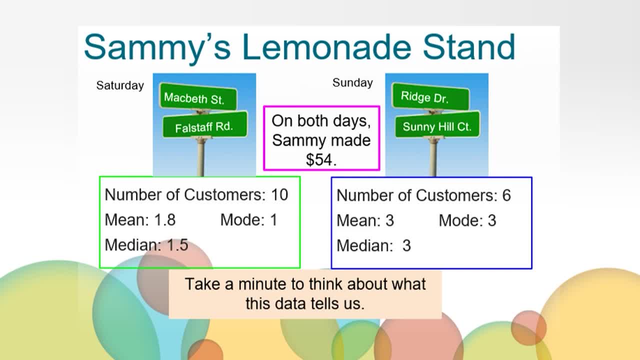 what they're looking for. We've got a new set of measures and standards. There's a positive model and then there's a negative. The negative will be set up by a professional. The negative will be selected by a team of experts. 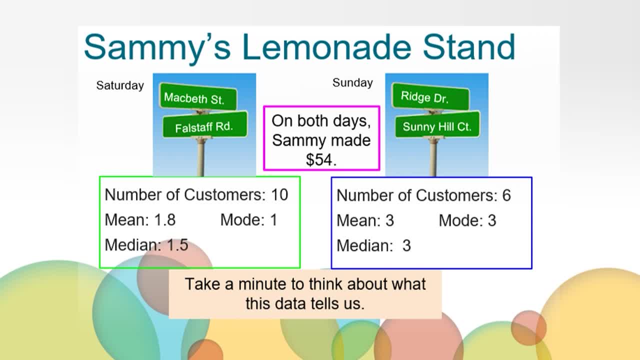 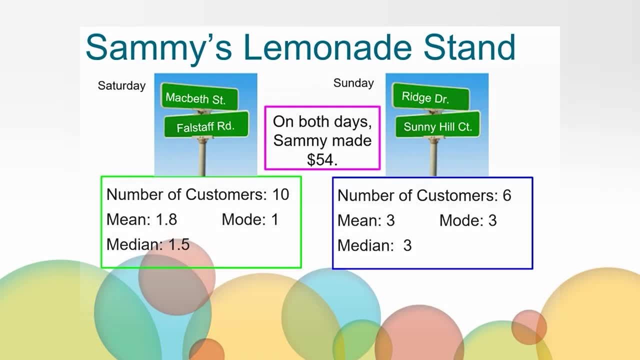 These challenges will be dealt with by a team of experts. It's going to be a tough job getting them to complete a specific task. So what does this data tell us? Well, on Saturday, there were 10 customers, and most of them bought only one cup of lemonade. 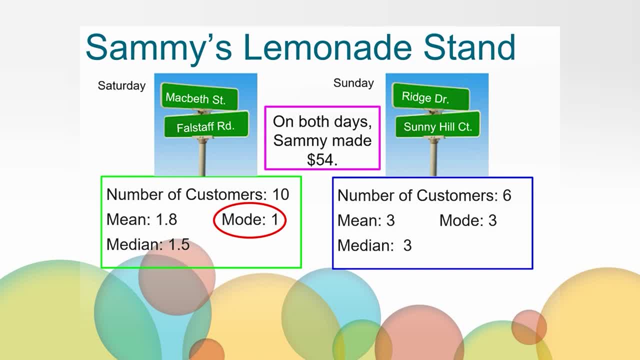 On Sunday there were fewer customers- only six- but most of those six bought three cups of lemonade. Both the mean and the median are lower on Saturday than on Sunday. I'm thinking this means that there are more people that stopped by the lemonade stand. 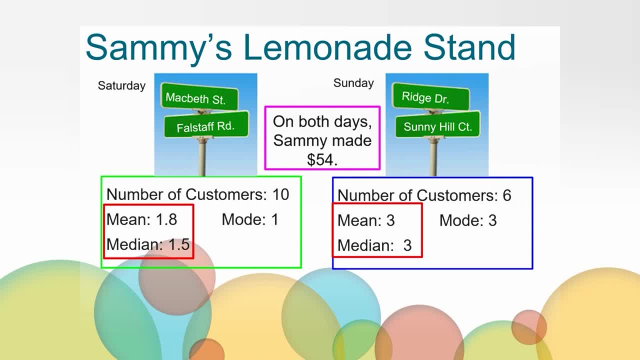 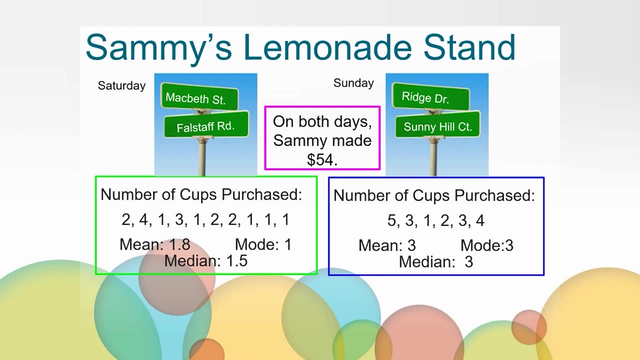 on Saturday who were by themselves On Sunday. I'm thinking that fewer people stopped by, but maybe they bought more cups for their family or friends who weren't with them. Take a look at this new information. You now can see the number of cups each customer purchased. 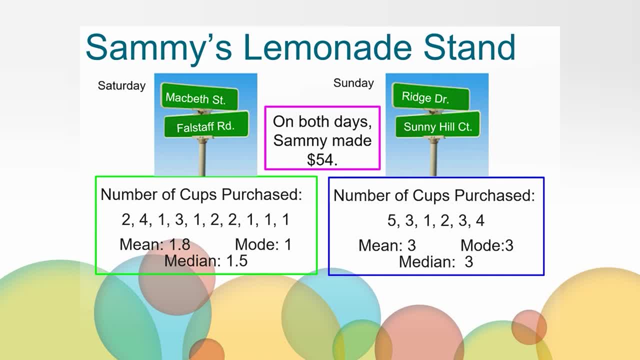 Were we correct in our thinking? In general, did more people buy fewer cups on Saturday than on Sunday? Yeah, on Saturday there were 10 customers. That's a lot of cups. That's a lot of cups. The first customer bought two cups. the next customer bought four cups. the next customer 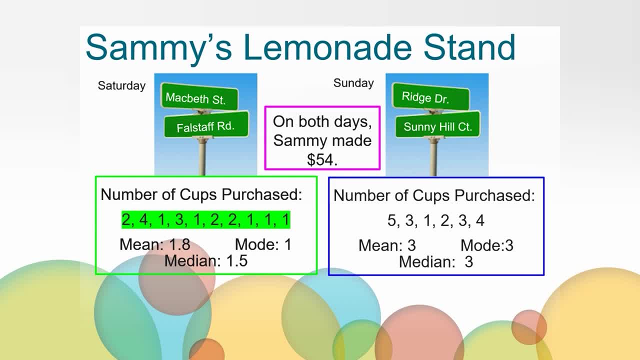 bought one cup, and so on, for a total of 18 cups. On Sunday, there were six customers who purchased a total of 18 cups. What conclusions can you draw from this data? How might it help you make a recommendation to Sammy about which corner he should set up? 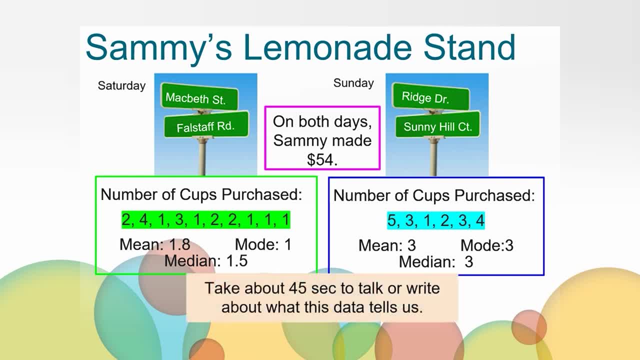 his stand next weekend. Practice being a communicator by sharing your thoughts with someone near you or by writing it down, Like this video, to help you understand the best way to set up your lemonade stand. At which corner do you think Sammy should set up his lemonade stand in the future? 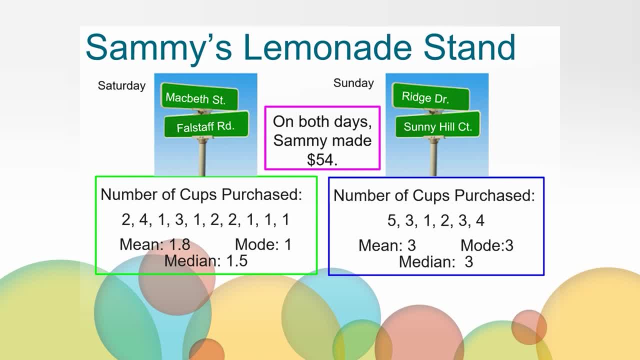 If Sammy likes staying busy and meeting lots of people, maybe the corner of Macbeth and Falstaff would be the best place for him. The data shows that more people went to his lemonade stand when it was at that corner than the other corner.